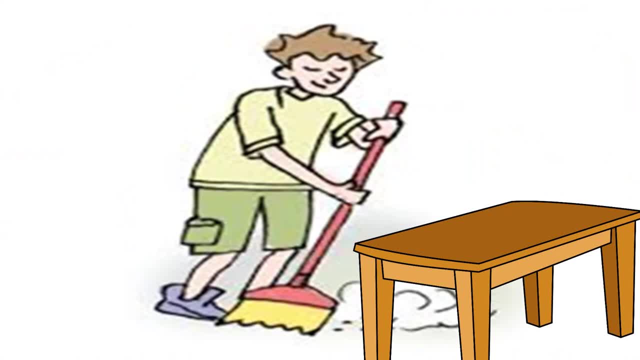 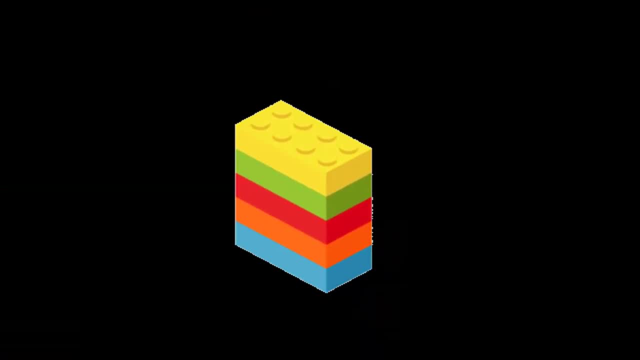 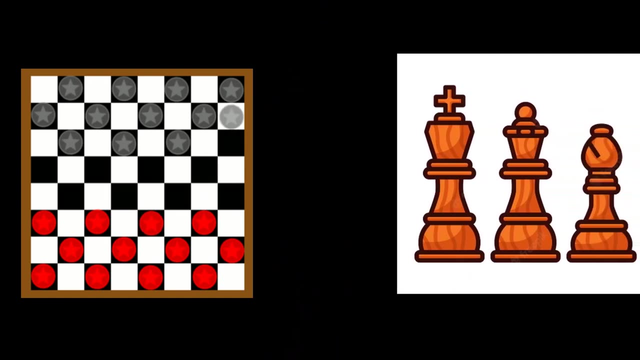 sweeping. you can ask the child to sweep under the table a block or lego game, or even laying down tracks is a great idea in which the concepts of front, back, top, bottom can easily be taught. games like checkers or chess, where there is specific orientation in which the pieces have. 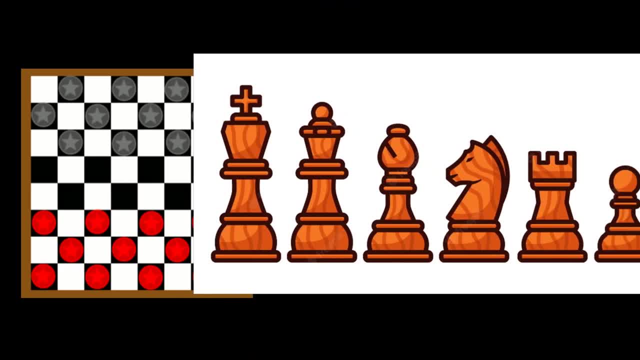 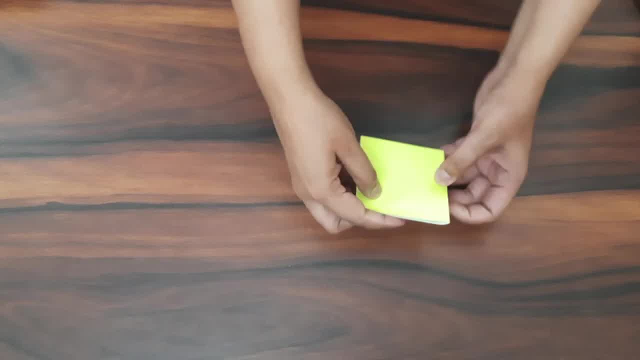 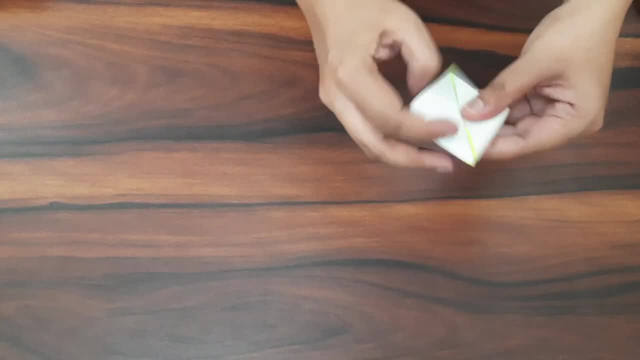 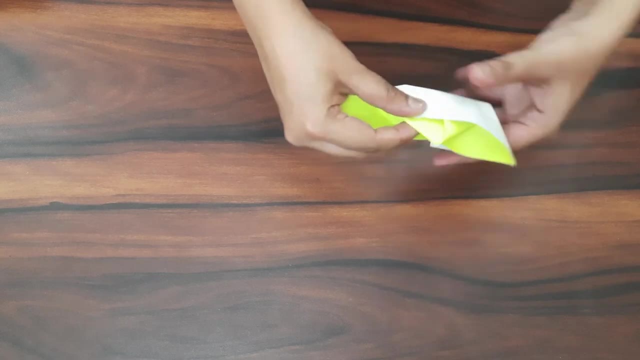 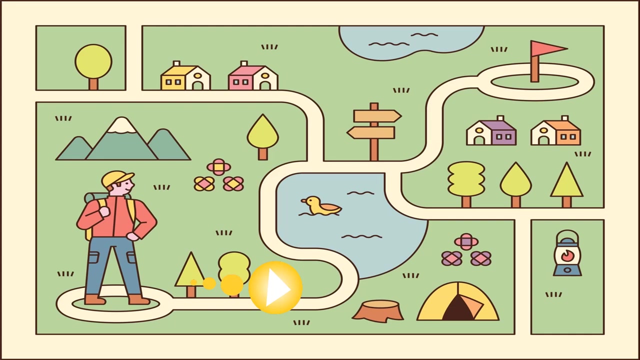 to move is a great way to teach spatial relations. different kind of crafts like origami, in which the folding has to be done, for example to make a boat, is another great way to teach spatial relations. if you have to try to direct the child to go maybe forward, backward, towards the left, towards. 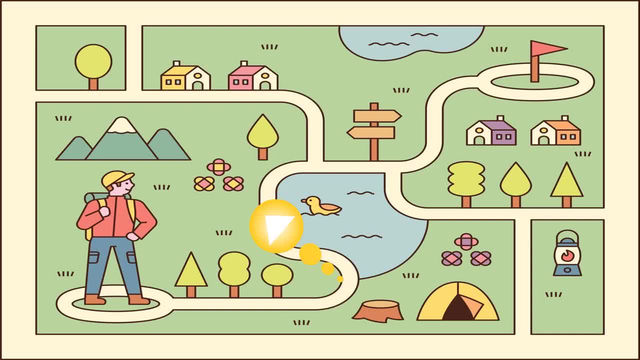 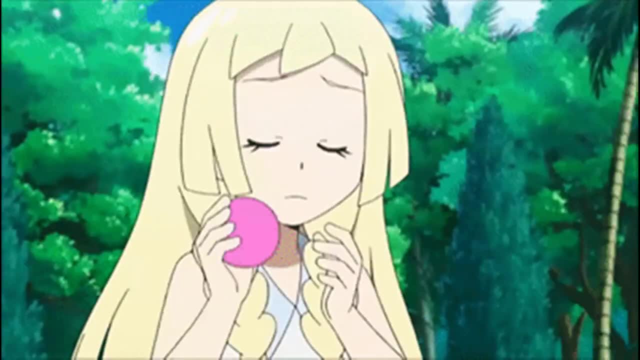 the right initially. Initially you can start with verbal as well as visual instructions, as in demonstrating to the child, and later on you can move to just giving verbal prompts for directions. Ball games are again extraordinary because if they are trying to shoot it towards a target, 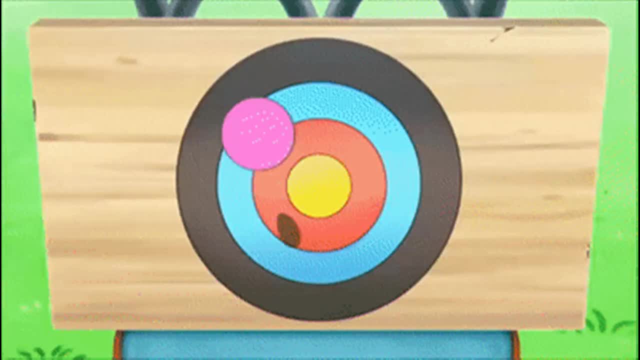 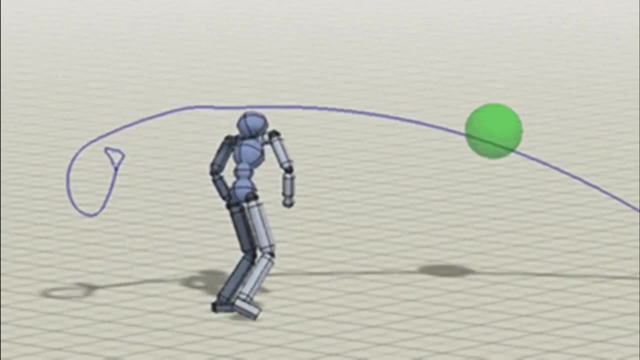 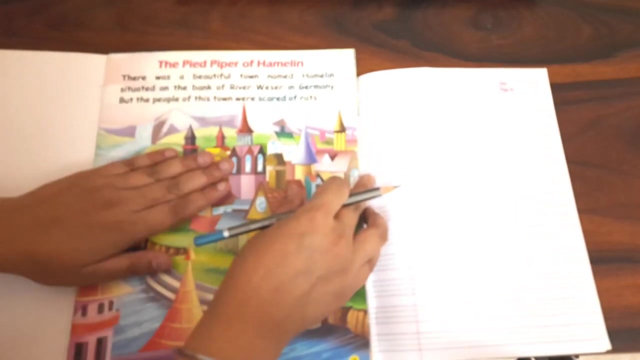 if the child is overshooting or undershooting, then, yes, child's spatial relation or the concept of visual perception is affected, also showing that their motor skills are affected. So that is an excellent game to play If a child is able to read or write without losing space, knowing that they always have. 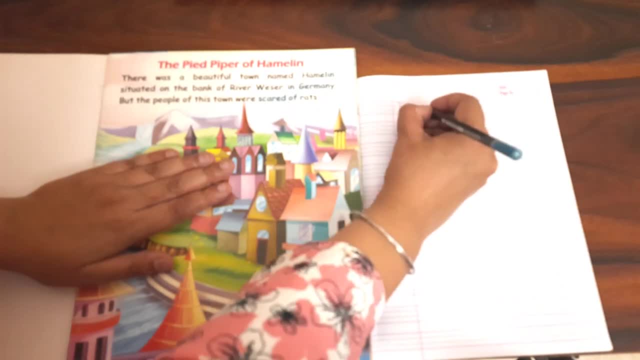 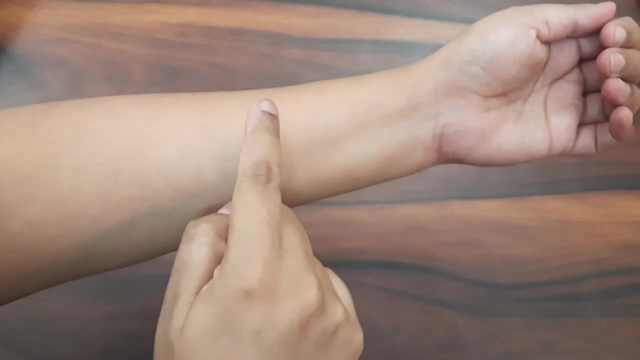 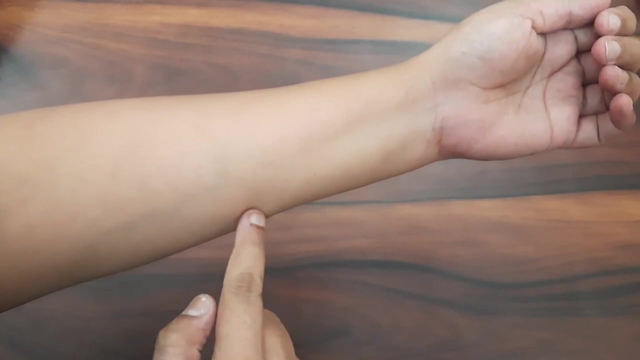 to come back to the left side in order to start reading the read from top to bottom. that is also spatial relations. A graphesthesia game is wonderful to play because in this you can ask the child what they want to see and the child will try to close their eyes and you can try to write. 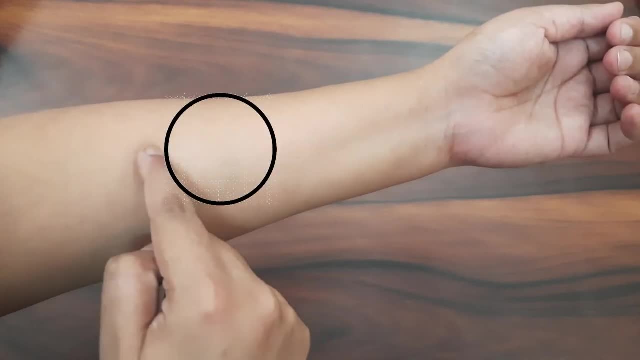 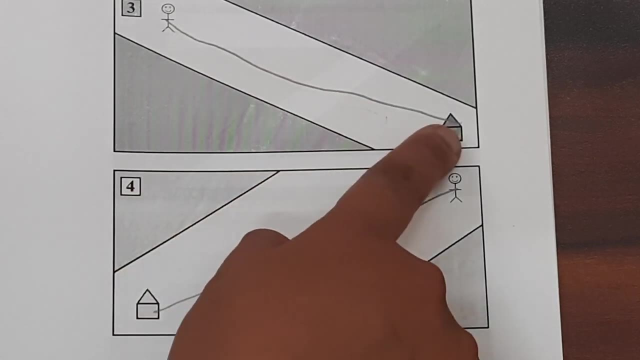 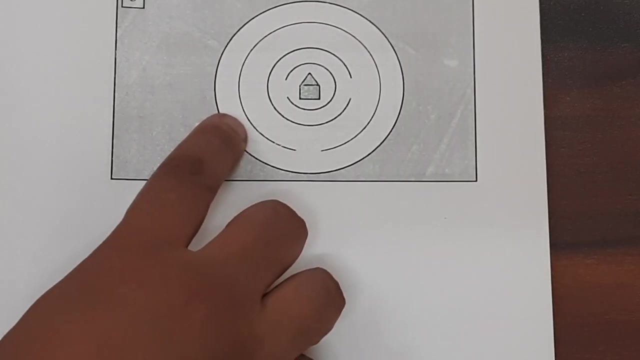 some alphabet number or draw a shape on their hand and they have to identify it. Mazes form another excellent way in which you have to go through making the mazes more complex, first starting with a basic straight line, then making it more curved, or you can. 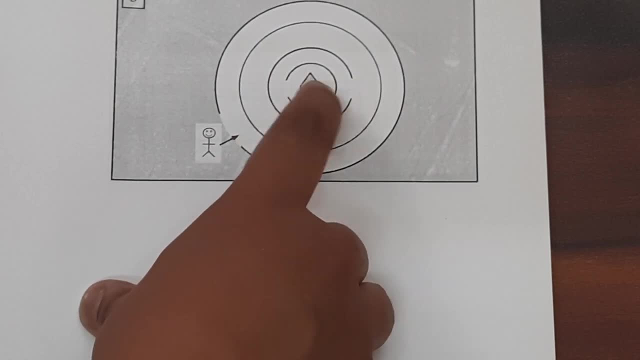 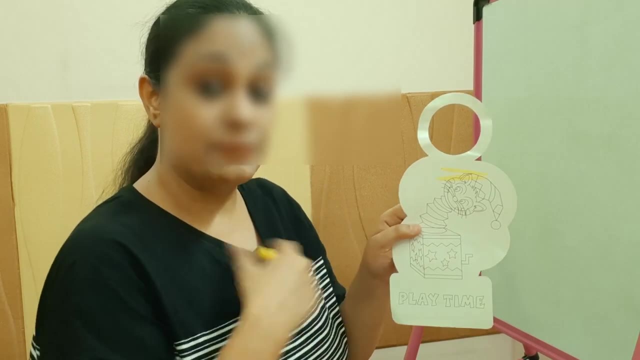 make it more complicated by making circular mazes for them. Coloring in complex pictures is again very important. Coloring in complex pictures is again very important. Coloring in complex pictures is again very important, Something that requires good visual spatial relation skills, as the colors may go out.